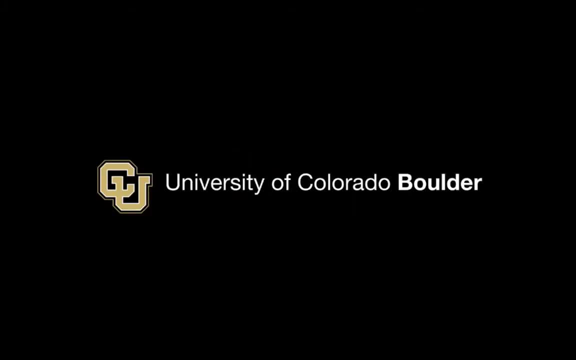 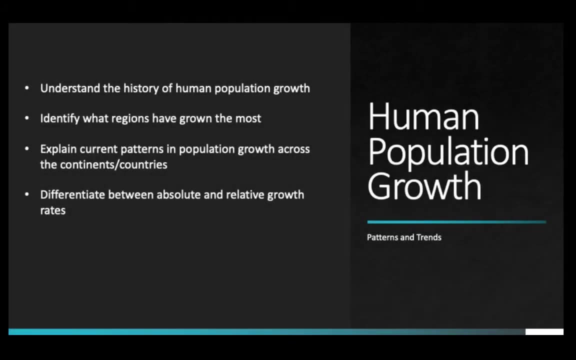 In this video we're going to talk about the basics of human population growth, and we'll start by looking at the history of human population so that we can understand when the human population started to grow and how much things have changed over the last couple hundred years. 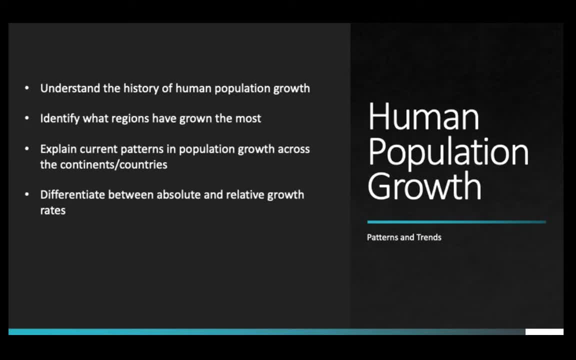 We're going to look at what regions have grown the most historically and look at patterns in population growth across continents and countries today As we move forward. this will provide a good foundation for understanding the future of human population growth. Lastly, we're going to talk about the difference between absolute and relative growth rates. 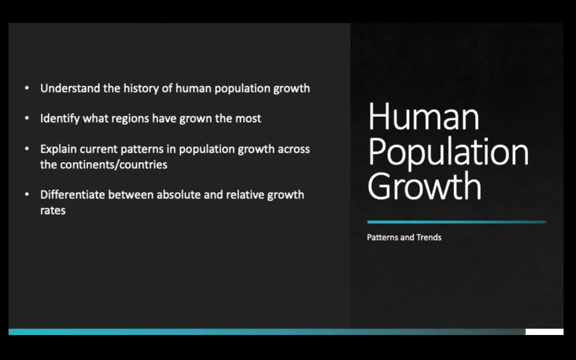 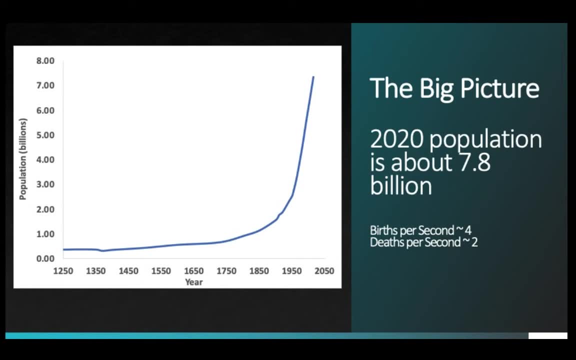 Understanding how these are different is really important to being able to predict how populations will change in the future. When did population really start growing? You can see the answer in this slide. For most of human history, there have not been very many people on the planet. 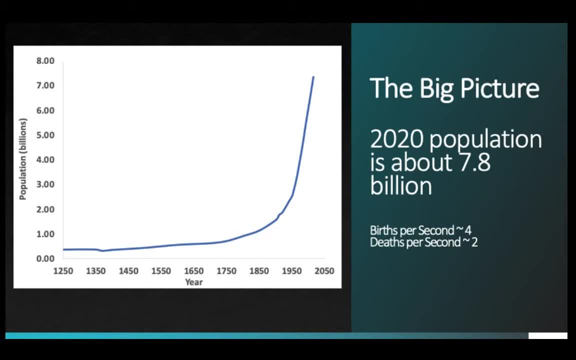 In fact, if we go back 600 years to the early 40s, there were only about 400 million people on Earth. We didn't hit our first billion until somewhere around 1880.. We hit 2 billion around 1925, 3 billion in 1960, 4 billion in 1975, 5 billion in 1988, 6 billion around 1997, 7 billion in 2011, and we'll hit 8 billion sometime in 2021. 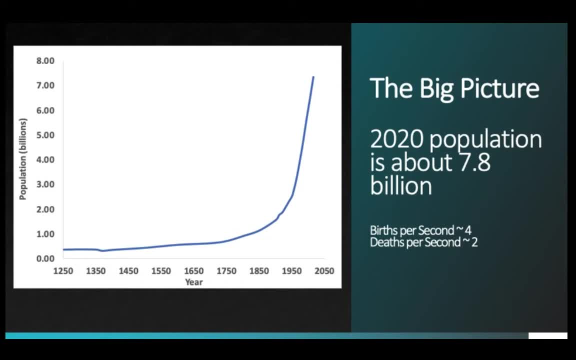 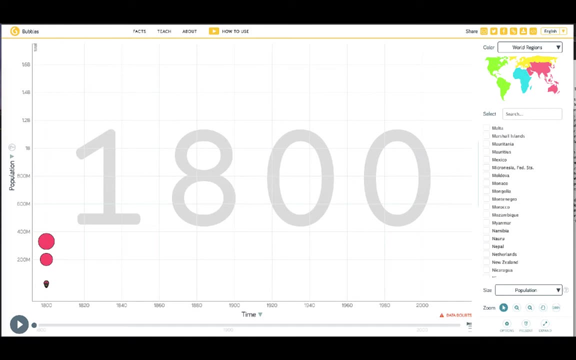 You can see the shape of this curve is a classic example of exponential growth, But there's a lot here. We can see what's hidden under this curve that we need to talk about to understand the future of population growth. Let's dig in a little deeper and look at how different countries have changed over the last couple hundred years. 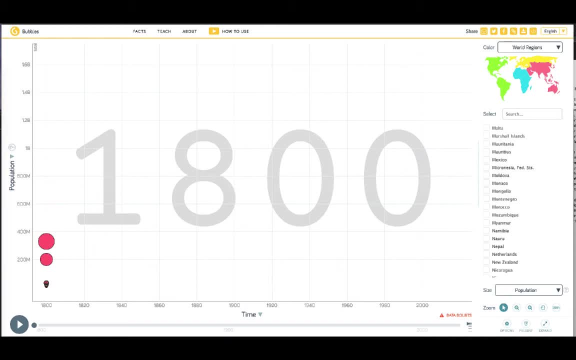 One of my favorite sites to use for looking at population data is gapminderorg, And the animations I'll show you here and in an upcoming slide are from that site. You can go to the site and explore a wide range of additional information around population, demographics and many other topics. 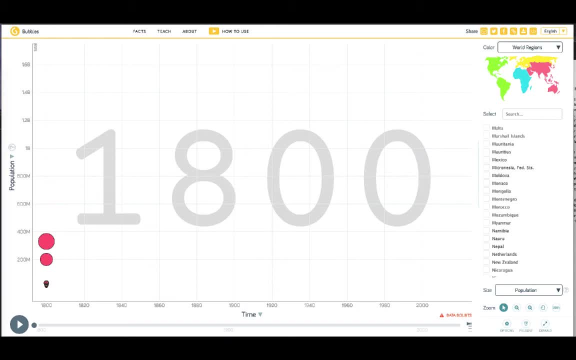 So let me orient you to this graph before we start. On this graph we see time on the x-axis, total population on the y, and each of the circles represents a country. The size of the circle is proportional to its population and the color of the circle tells you what part of the world it represents. 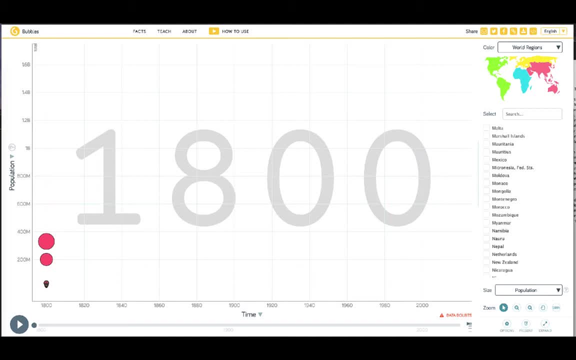 Red for Asia, blue for Africa, yellow for Europe and Russia and green for the Americas. Those two big red circles, you see, are China on the top and India just below. The entire rest of the world is in those little dots at the bottom. 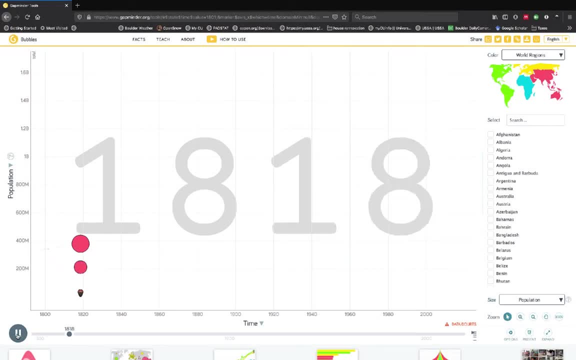 As we watch this animation go forward, we see a lot of things change. First, China was a big country to start and it gets bigger as time goes on. India is also large and the two together dominate world population up to about 1900.. 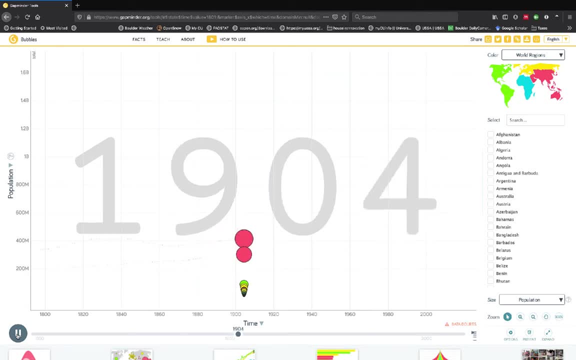 Then things start to change a little bit. That green dot that starts to emerge in the 1920s is the United States and you can see it will continue to go up By the end of the curve. you can see that China's growth takes. 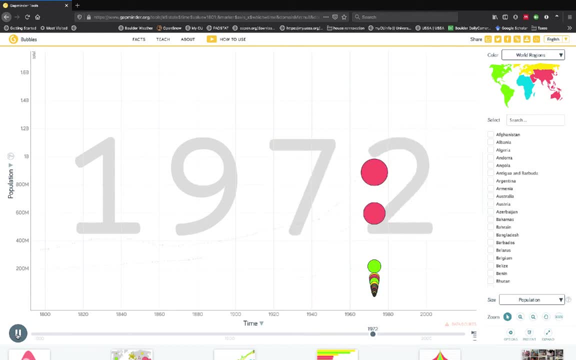 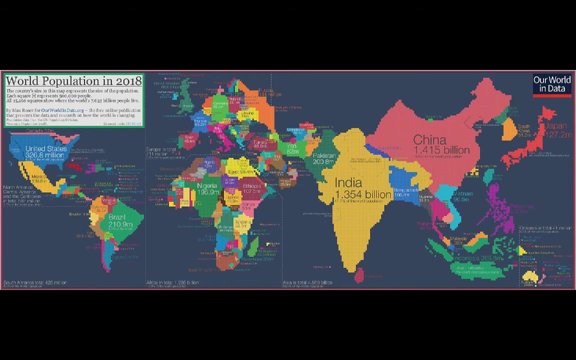 off in the 70s and 80s, and that brings us up to where we are now. The next image shows us what world population looks like in 2018.. Each little square on the map represents a half million people, and the size of the country gives you a sense of the total population. 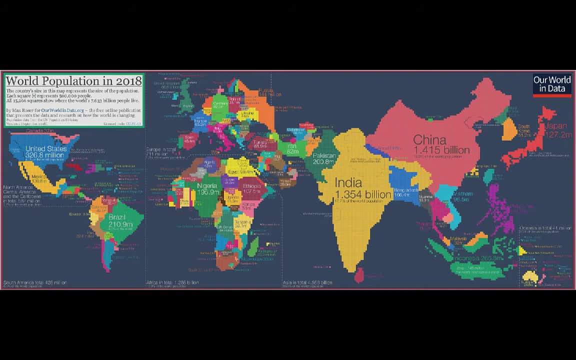 China and India are the largest countries in the world. One interesting thing to note on the top is how many of the world's most important economic powers really do not have large populations. Look at the European countries for an example of that. Now notice that many of the poorer countries on the planet, particularly those in Sub-Saharan Africa, Indonesia and parts of Asia, 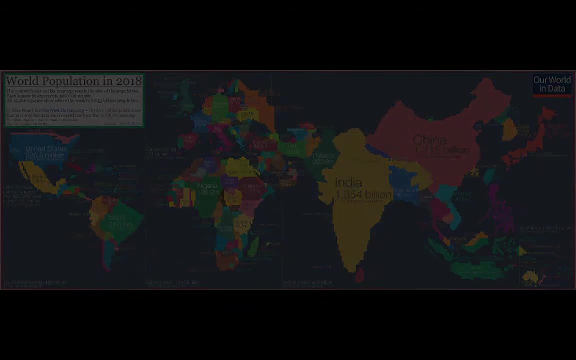 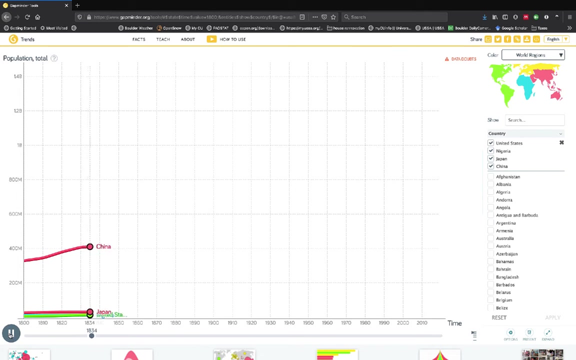 also have very large populations. Now let's take a look at how four example countries have changed over time. The US and Japan are wealthy industrialized countries. China was a poor country through much of the 20th century, but that has changed over time. 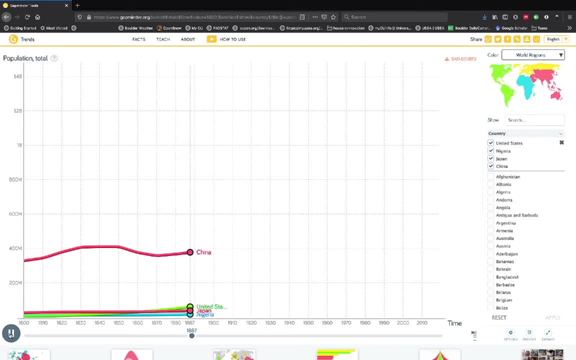 And Nigeria remains a low-income country today. Let's look at each one of these countries separately, as the image progresses. China's population started to rise quickly around 1950, but, as you can see, the curve bends downward around the mid-1990s. 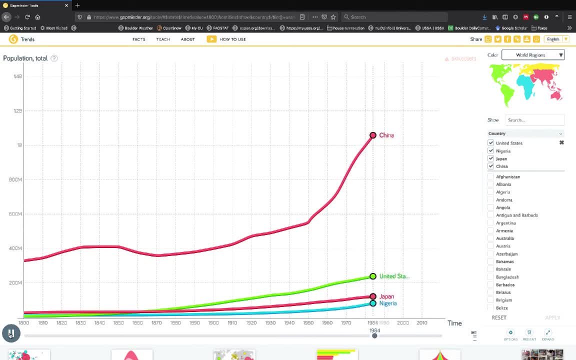 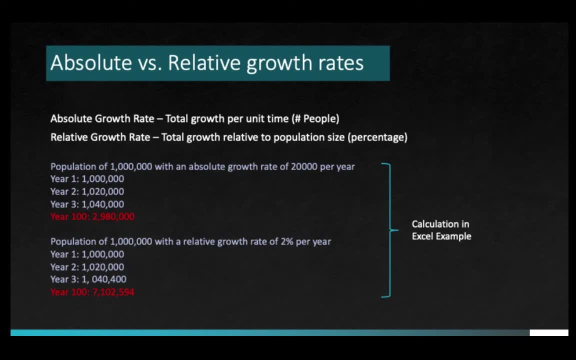 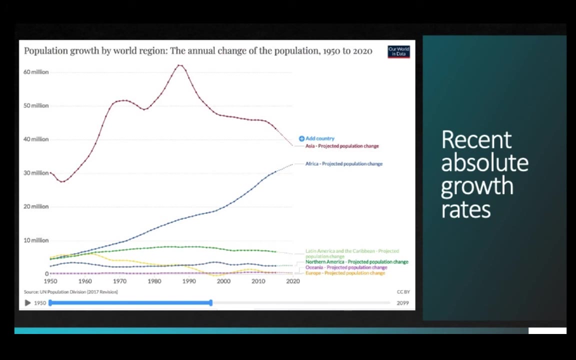 that's 20,400 people, And by year 100,- we reach over 7 million people. This is an example of what's called exponential growth. If we now take a look at absolute growth rates around the world, then what we see is that Asia has the largest absolute growth rate, but that 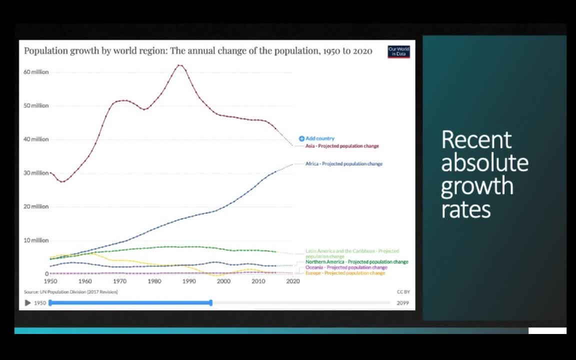 it has declined over the past 20 years. Now, keep in mind that Asia is also the most populated part of the world, and so it makes sense that a bigger population will have a larger absolute growth rate, even if the relative growth rate is low, as we'll see on the next slide.